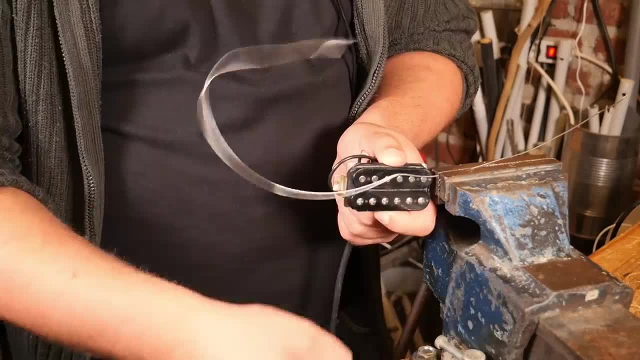 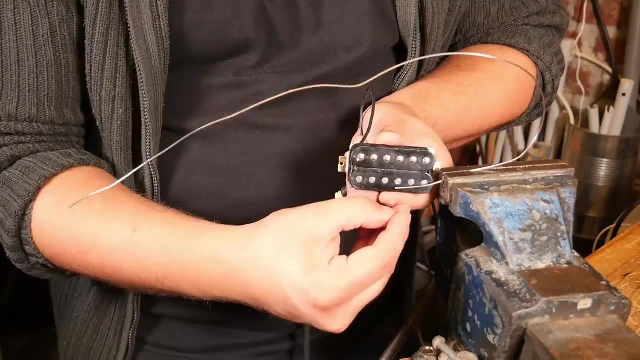 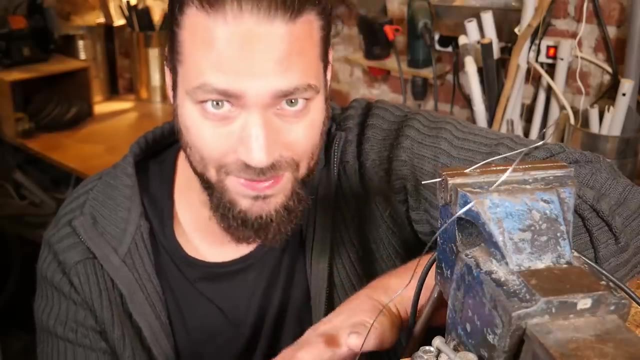 sounds with a lot of overtones And the small ones sounds like a crystalline Sansa. There is so much crazy sounds with this piece of metal. Before building my instrument, I need to make a device to deep sample the sound. I'm going to use a guitar pick. I'm going to use a. 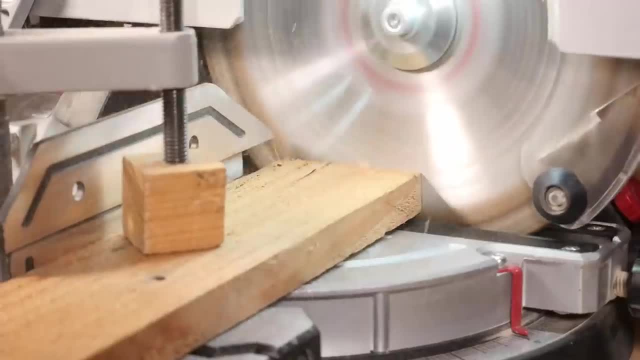 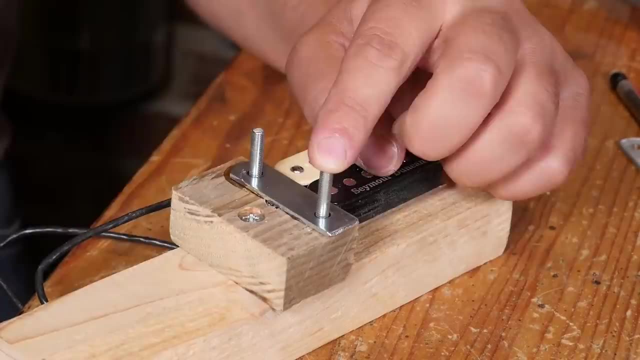 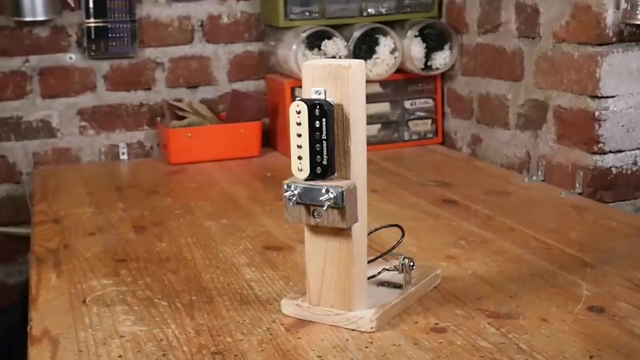 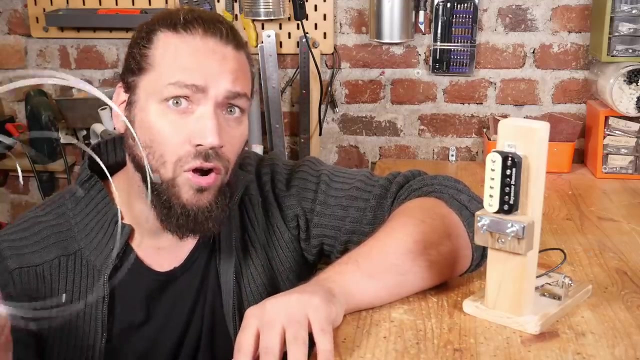 guitar pick and I'm going to sample this. The device is finished. Now I will need around 10 hours of deep sampling to record all the strings. I will be on tour in a few days and this is the perfect instrument to sample in a quiet hotel room. 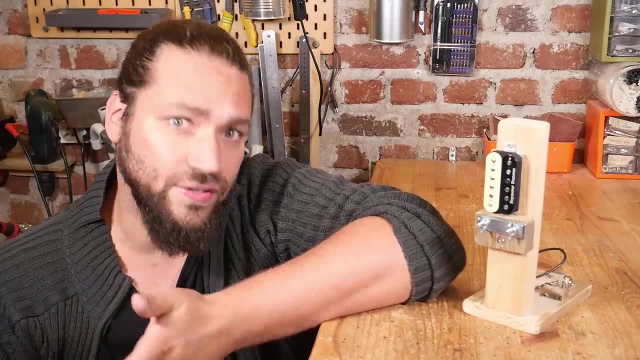 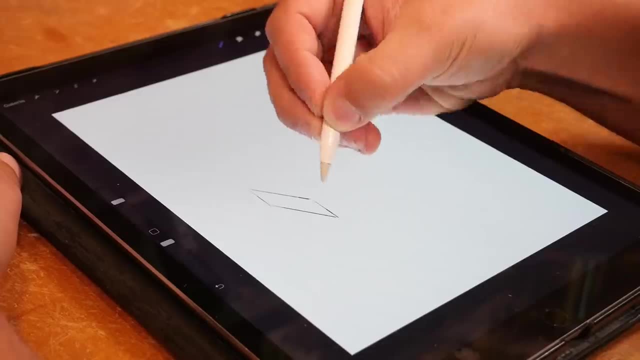 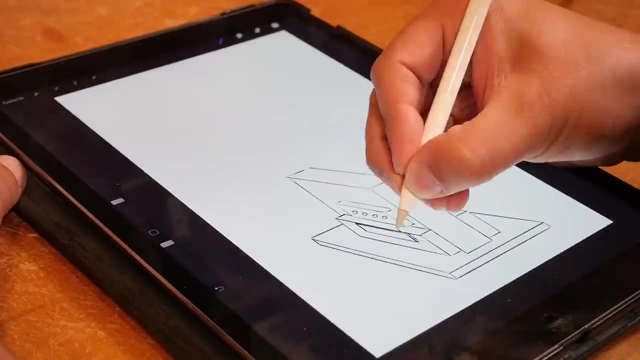 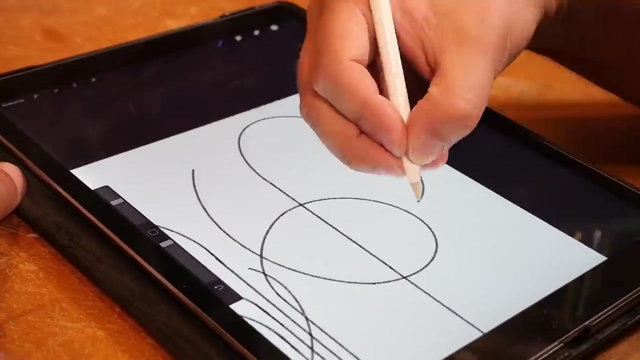 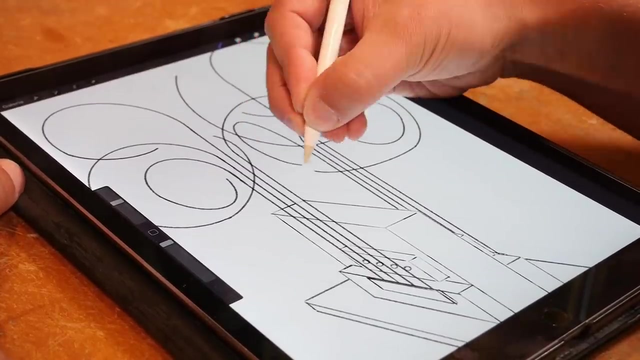 I still have one full day in my workshop, so let's design this first idea For this instrument. I want to use those two bass microphones. This will be an eight-nose notes instruments. I don't know if I will be able to tune those roads precisely or if it will be more like 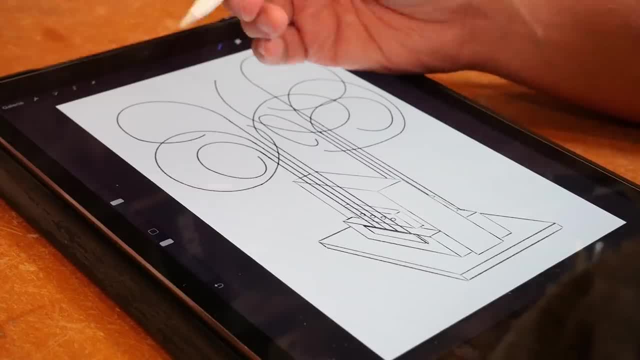 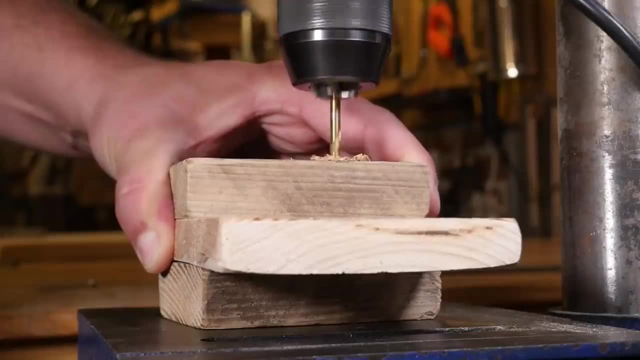 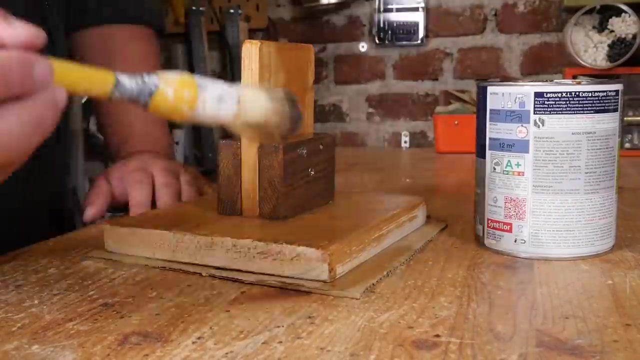 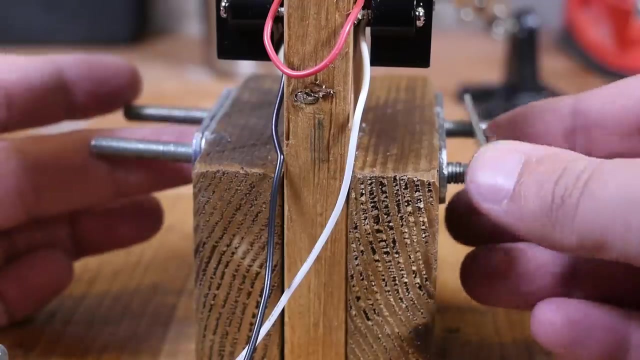 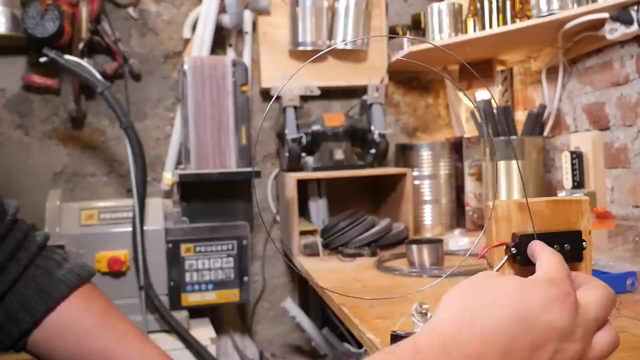 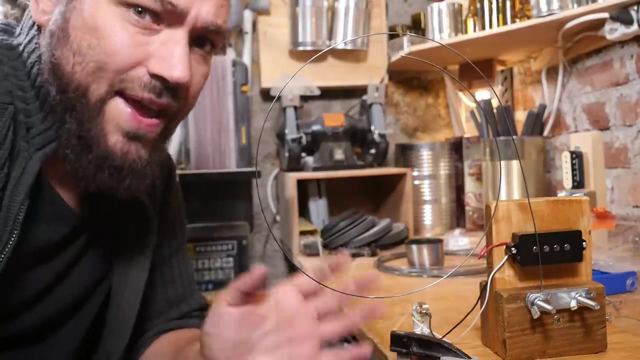 a sound sculpture. I will take my time to tune each one and we will see Impressive woodworking. I will varnish it this time. First string. I will put the 7 other ones with random length and try to find a global shape. 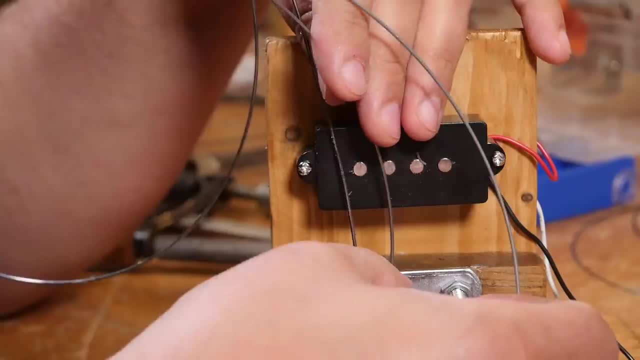 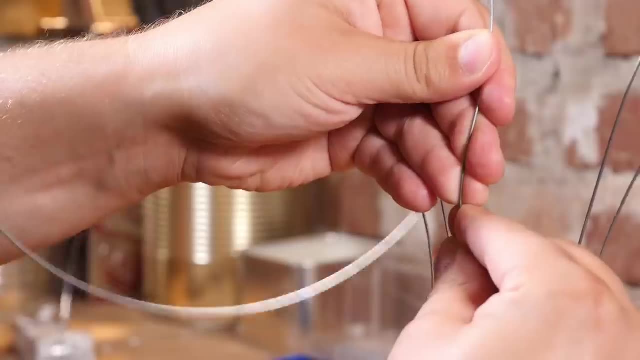 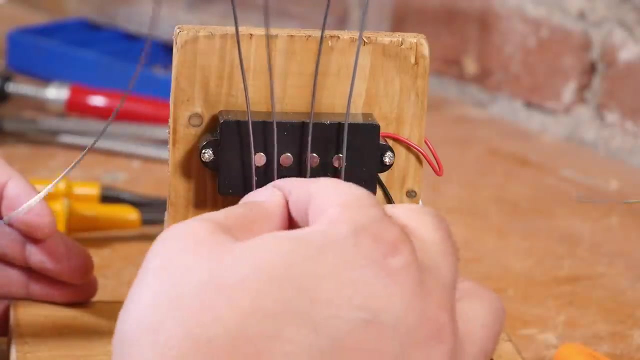 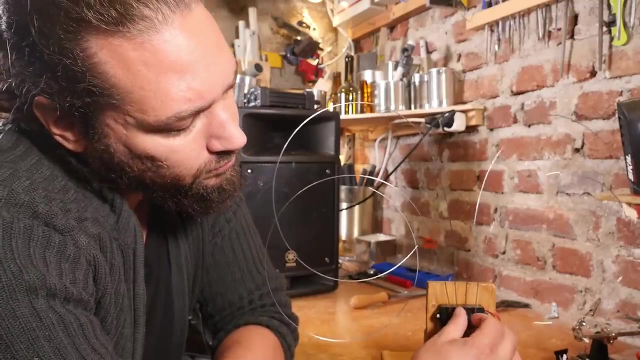 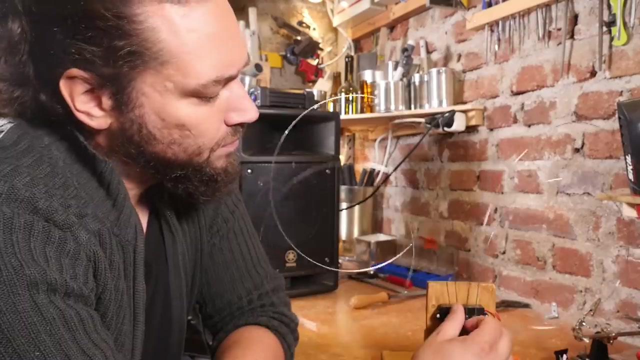 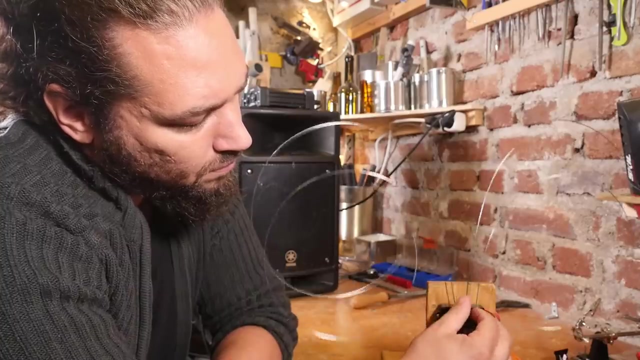 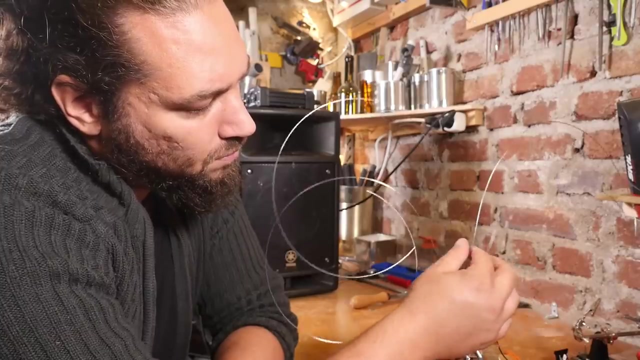 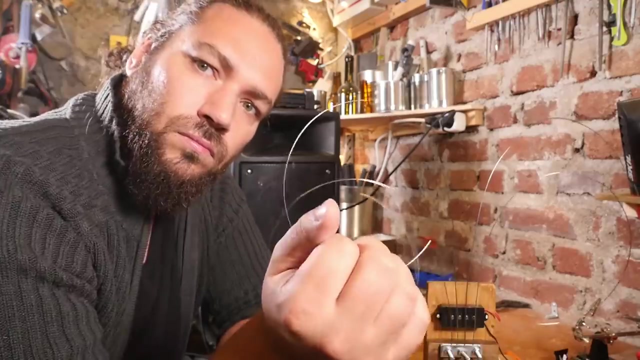 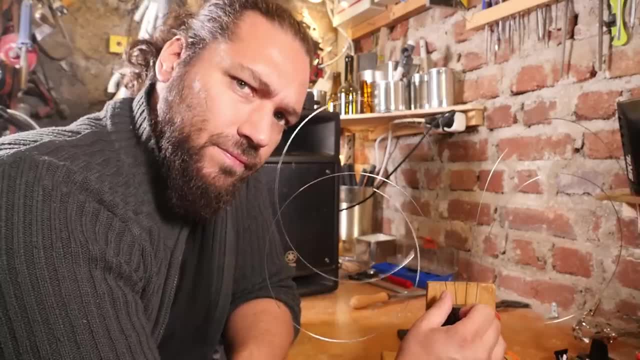 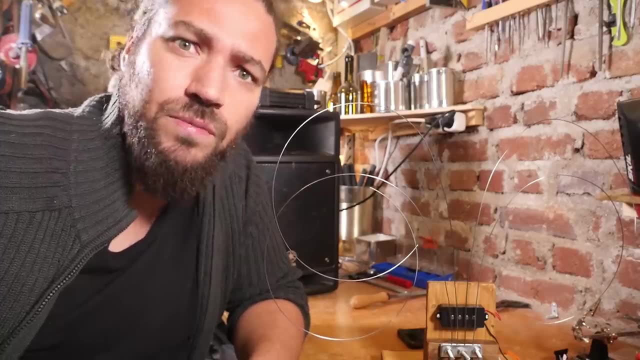 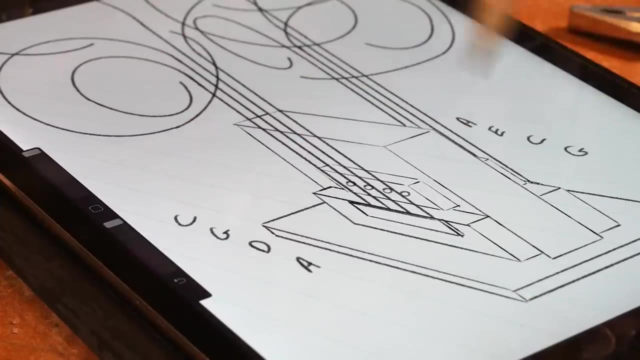 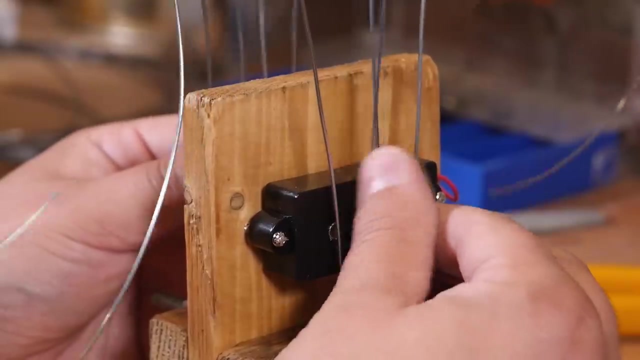 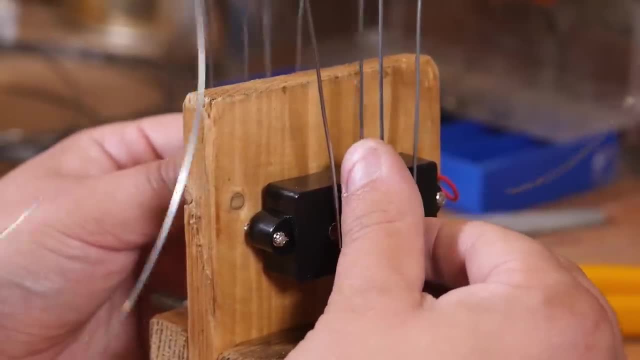 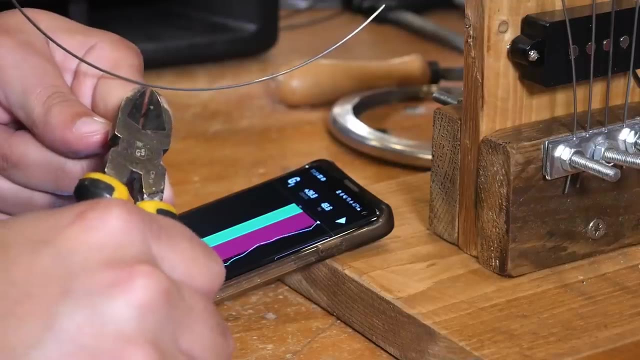 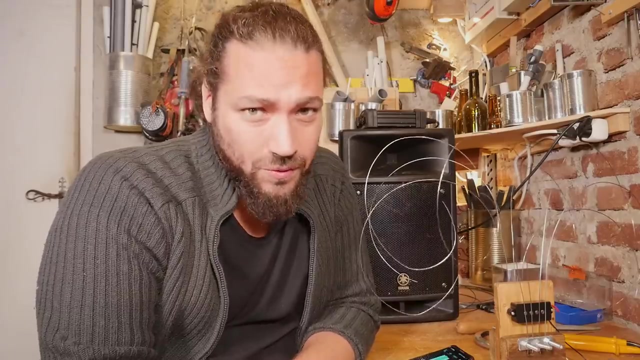 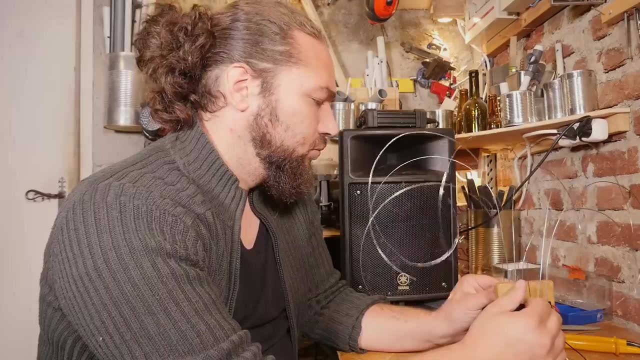 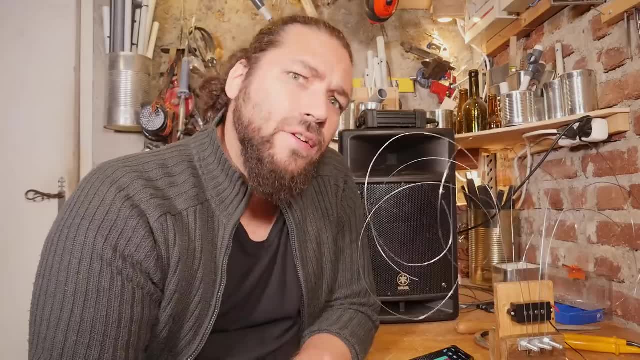 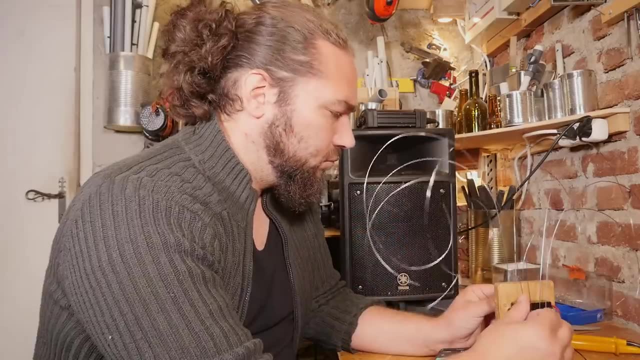 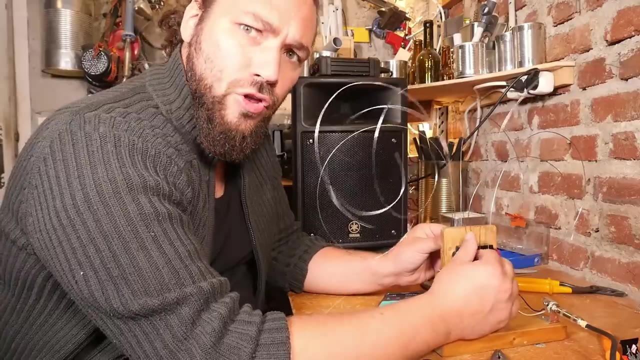 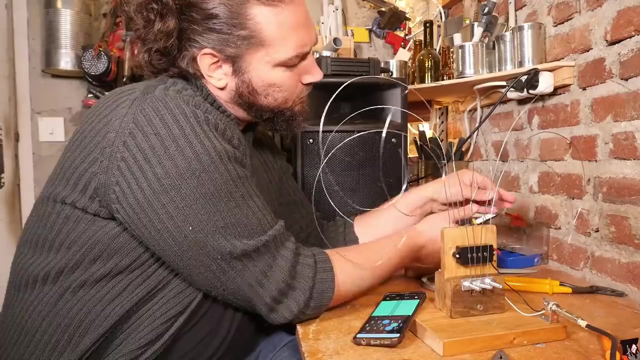 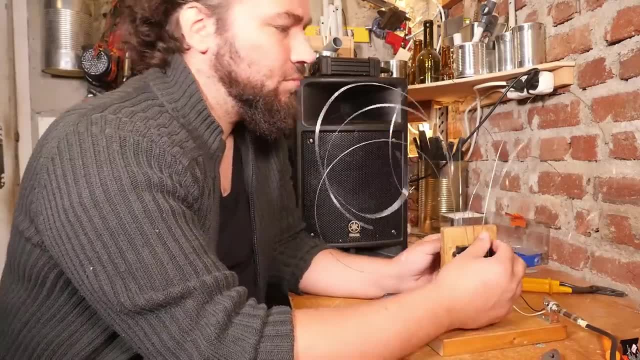 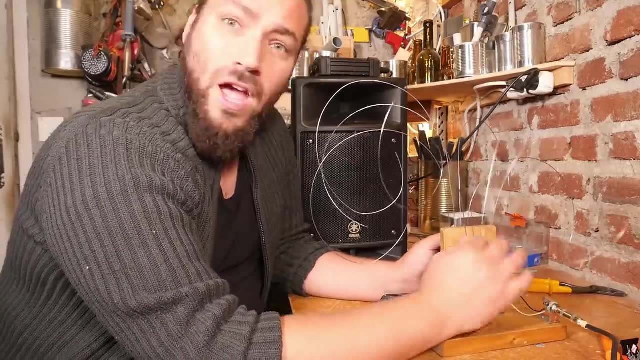 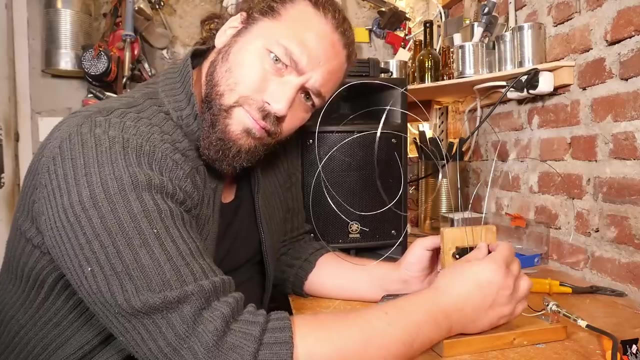 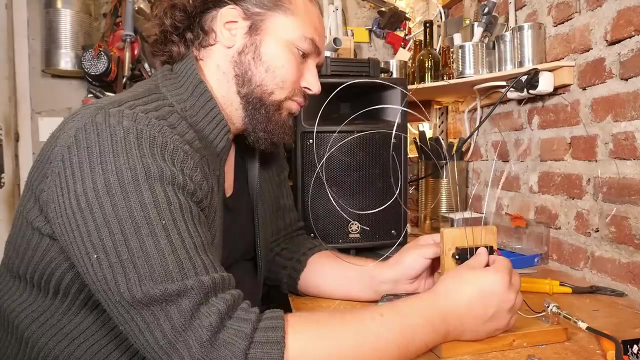